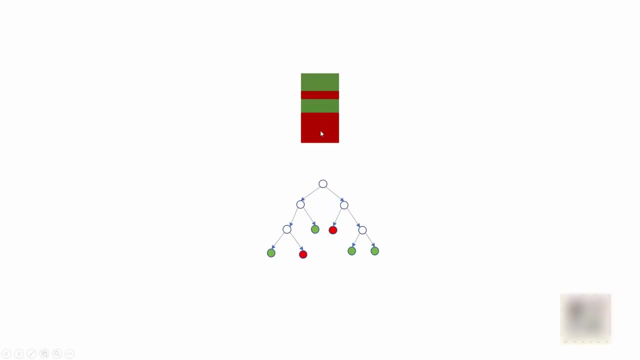 there you have it. You have green samples, red samples and based on that, you build your decision tree. Now, how can you build multiple decision trees out of this single data set? Well, one approach is: you build a decision tree and then you build a decision tree. Now, how can you build? 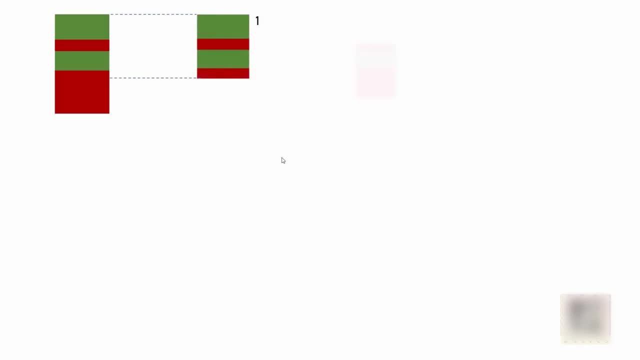 multiple decision trees out of this single data set. Well, you take your data set, then you divide it into a batch of random data sets, then you build decision tree for each of them. So, since we did random sampling here in random forest and now we have multiple trees, so you see a forest being formed already, Once it is trained you. 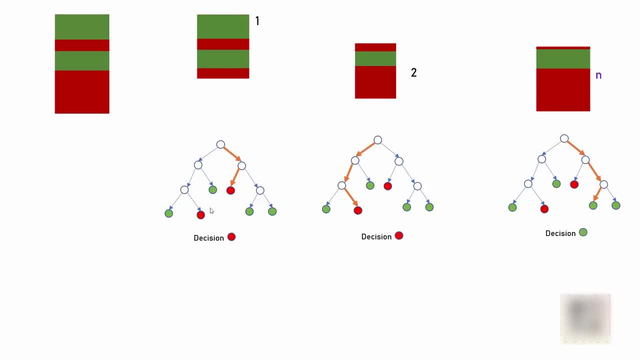 give the thing that you want to predict and they will all come up with different decision. You just and get a decision. so this is the basic crux behind the random forest algorithm, and i recently used similar approach to make a decision in my real life. i wanted to buy this thermostat and i 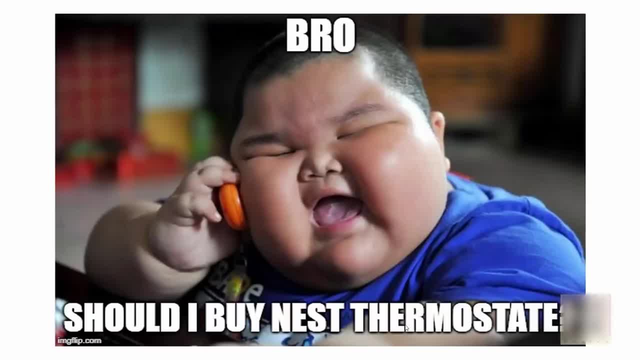 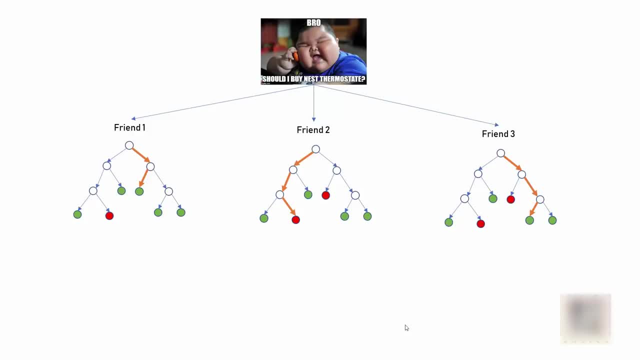 called bunch of my friends- and yeah, by the way, that's me in the picture- and those smart dudes gave me different opinions. one guy told me: you know, it's gonna save you so much money- i saved like 500 last year- so you should buy it. the other friend say: oh, it's freaking 200, it's a waste of. 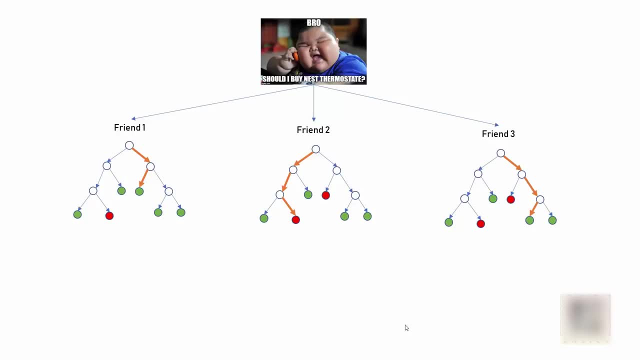 money, don't buy it. third guy told me: oh, you can control your temperature remotely anywhere from outside, so definitely buy it. all i did is just took a majority what? and decided to buy it. see, making decisions is so simple in life. just call your friends and take a majority. war, all right. 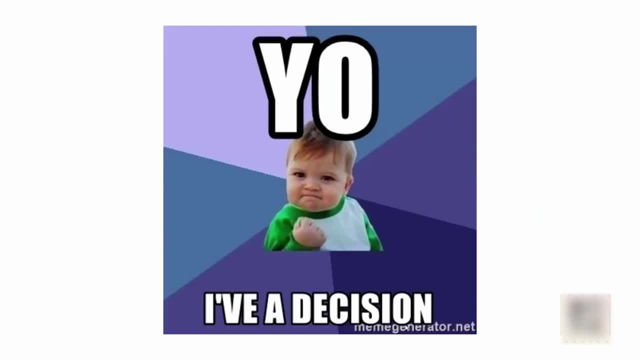 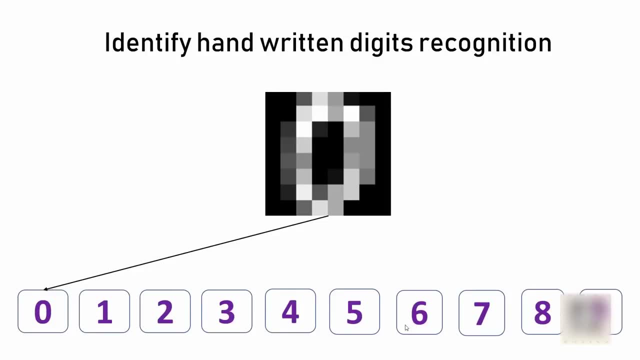 it doesn't work all the time, but at least in this case it worked and i had a decision, and i'm not making this up, i just installed it yesterday. all right, now we're going to use sk learns digits data set to make a classification using random forest, so that data set basically contains the images of handwritten characters. 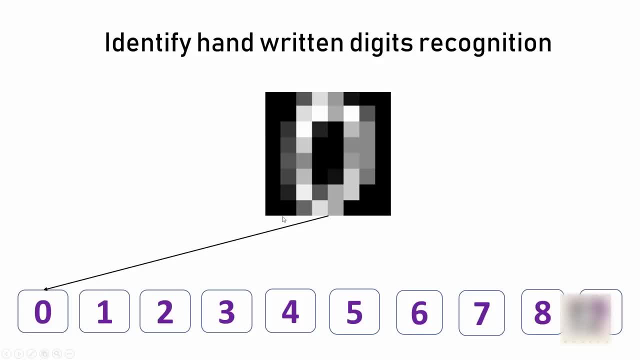 and all you're trying to do is just classify into one of these 10 categories where there is a digit from 0 to 10, and then you're going to use the data set to classify into one of these 10. all right, so that's what we will do in our python coding today, and in the end we will have an. 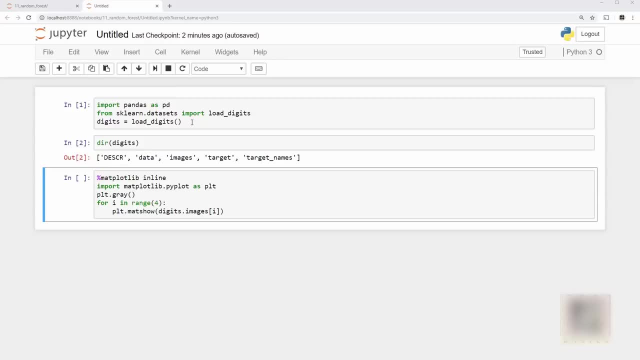 interesting exercise for you to solve. as usual, i have launched my jupiter notebook and loaded the digits data set from sk learn. data sets all right, and if i look at the properties of this data set, it has the real data and the target. all right, now i'm going to use matplotlib to visualize. 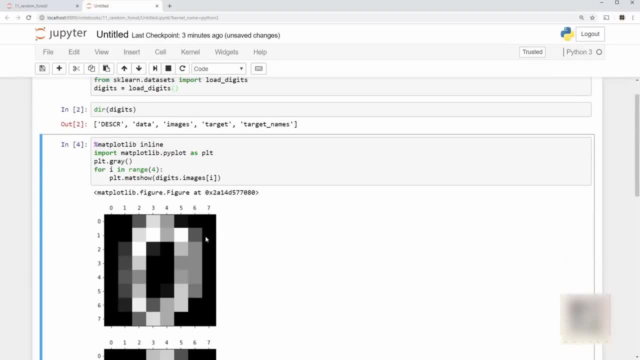 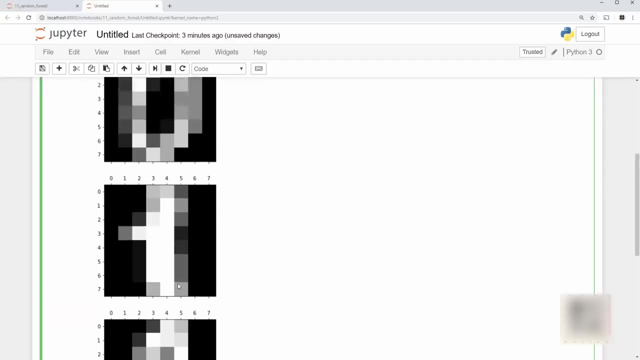 and when i run this, it looks like this. so i have basically handwritten characters, which is like 8 by 8 pixel array, it's like a multi-dimensional array, and when i use matplotlib it looks like this. you can see: this is character 0, 1, 2, 3 and so on. okay, now i will create a pandas data frame. 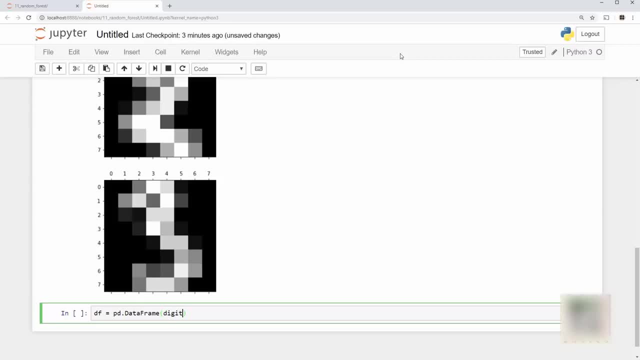 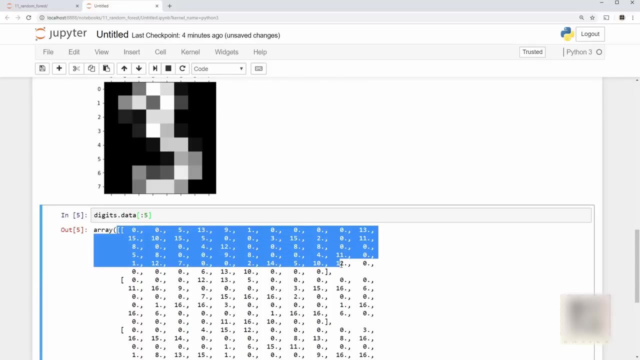 from this data set. so digits, data, basically data is if see, if you want to see it, just to make it simple, you will see that it is a two-dimensional array of numbers. so let's look at first five. see first five. like each element is just a two-dimensional. 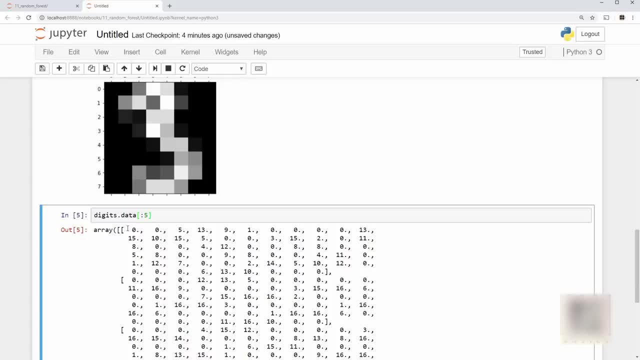 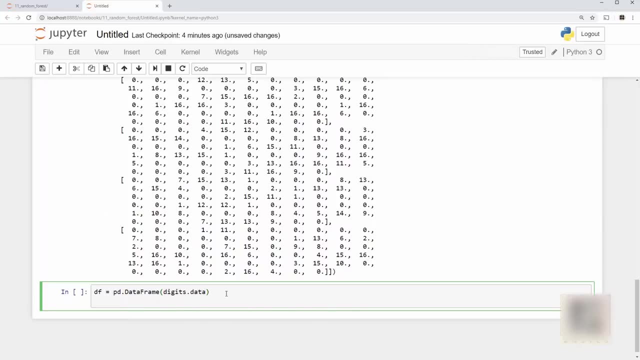 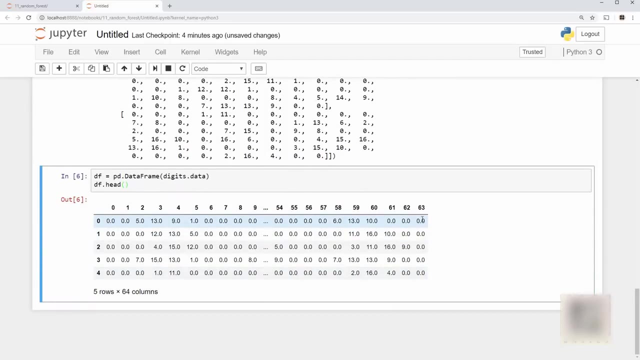 it's. it's actually one dimensional array, but it's like eight by eight metrics, so the length of this array is 64.. okay, and you can visualize this in a better way if you are using data frame. each sample is nothing but an array of 64 integers and they map to the 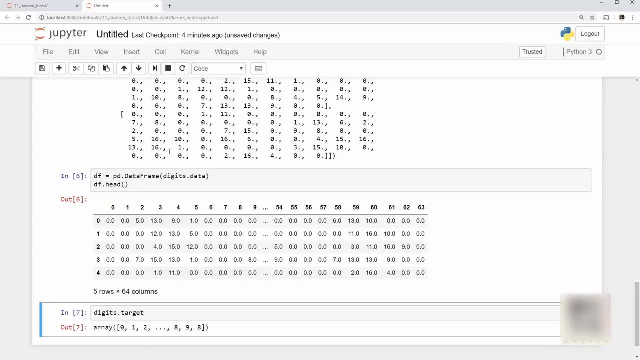 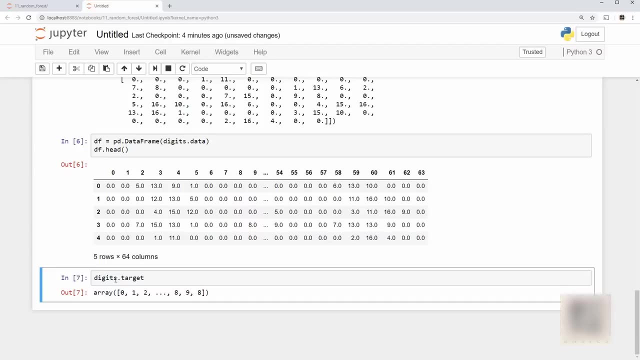 target variable. so if you do digits dot target, it is showing the target variable and i'm going to append that to my data frame. this is how you create a new column in pandas data frame. this is nothing but digits dot target. and when i look at my df dot head: 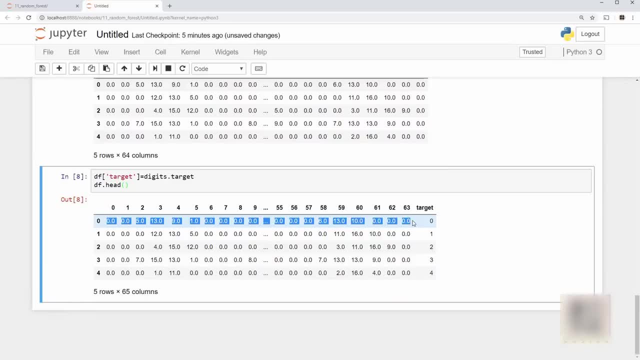 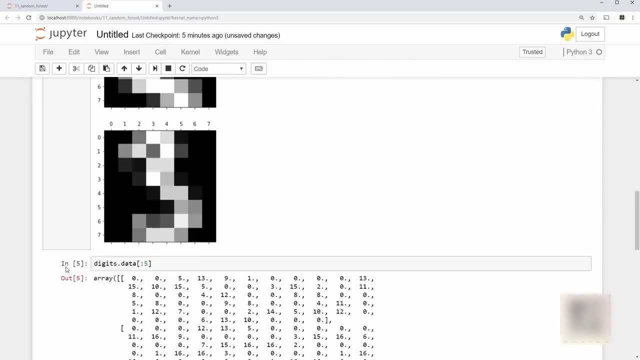 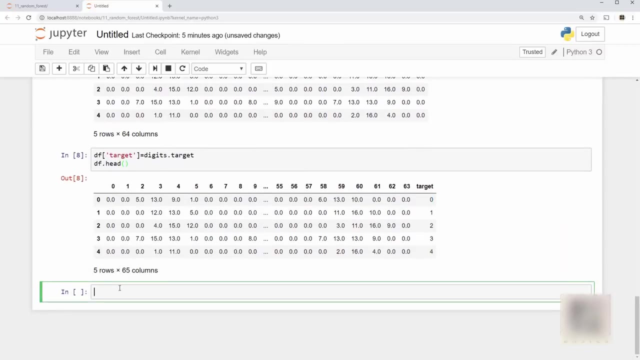 it says that this 64 uh samples they map to zero. all right. so, for example, this picture here is actually zero. so this target is showing you the truth. all right. now what i'm going to do is use train test split. i will do from sk learn dot model selection. 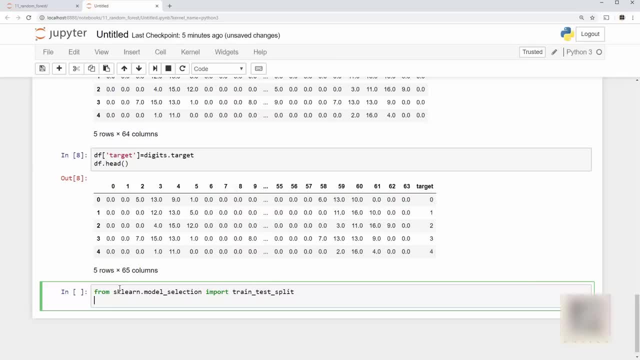 import train taste split. once you import that, you need x train, x taste, y train, y taste, okay and train split, and so your df and f and stuff like that. now you are on this fallait um, so you know it's simple to get the gears. i have all these elephant throughout here. 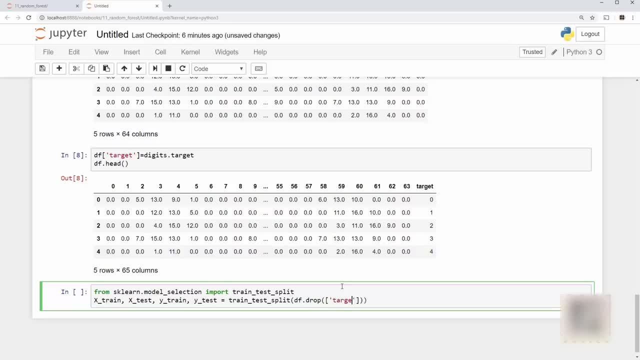 so let's go ahead with thisihad and test, set it up with bus and dear on this, use nights, Puis, and you can do. includes them with these buttons here. oh, if you wanna move how you want to split your training and test data, when I say test size equal to, 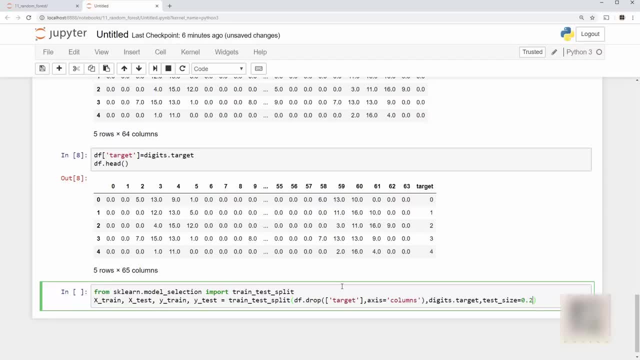 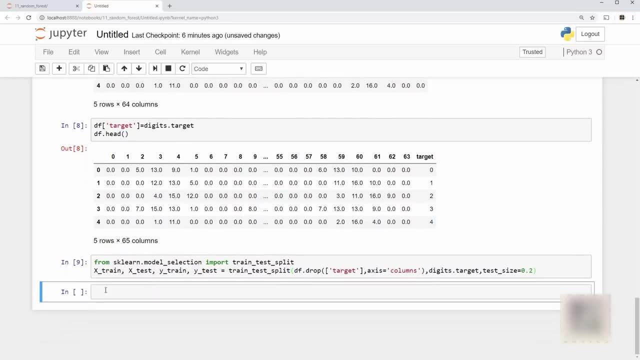 0.2. it means 20% of my sample is test data and 80% are training. okay, when I run this, it created all these four variables and when you look at size of your x-train, it is 1437 whereas x-test is this. so this means 20% of your total. 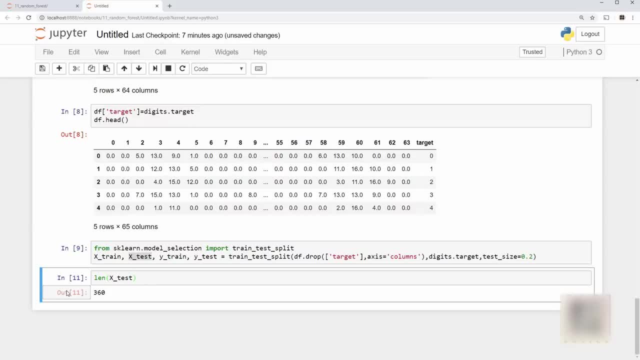 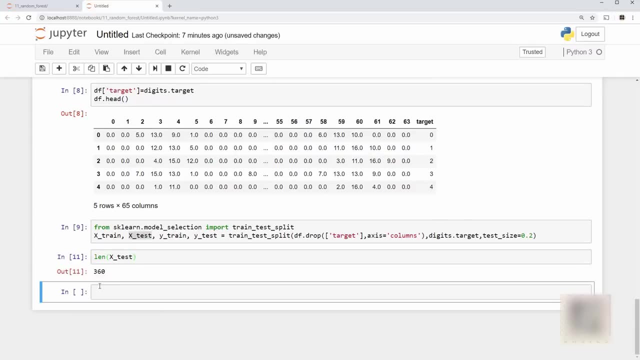 samples. so now I have nice training and test samples I can use. now the random forest classifier are to train my model. alright, so from sklearn dot ensemble. now why is it called ensemble? ensemble is a term used when you are using multiple algorithms to predict the outcome. all right, that's what way we are doing here. we are building multiple. 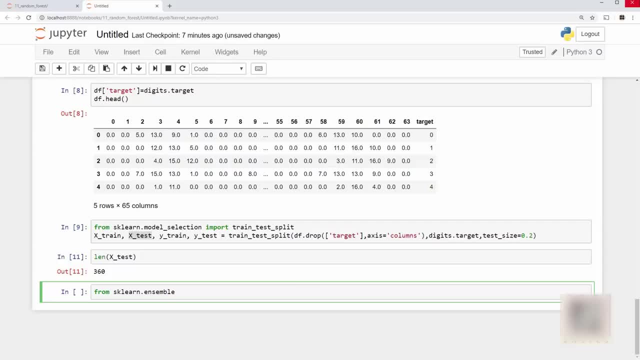 decision trees and taking a majority, what to come up with our final outcome. so that's why it's called ensemble, from that import random forest classifier, okay, and then just called model-dot fit ruby-ohmouth. this is your training step. after this step, your models will be trained and it trains the model and you can see bunch. 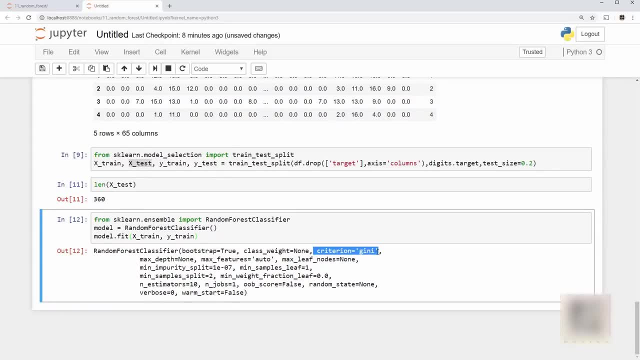 of parameters here. so the genian entropy criteria is something that you studied in the decision tree tutorial already, so that's what this is. you also have estimators. so here, 10 means it used 10 random trees, okay, and we are going to see the performance using. 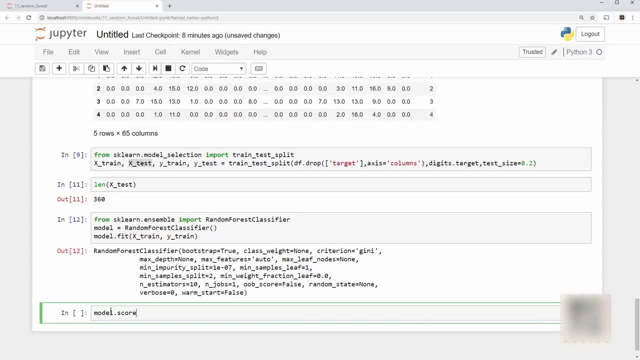 the 10 random trees. so let's call modelscore on x taste and y taste and we can see that the accuracy is 91. okay, when we use 10 random trees, the accuracy was 91. now let me try to tune this model and by and by giving 20 random trees, so i train it using 20 trees. 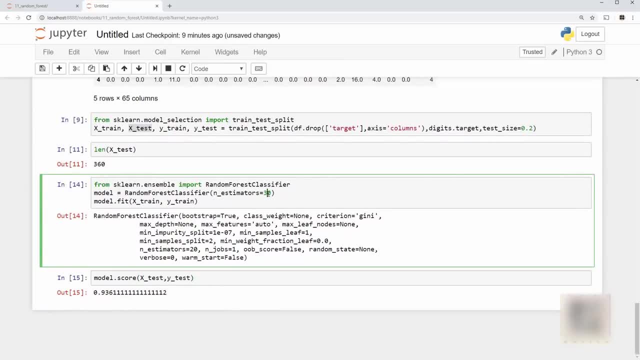 you can see my score is increasing. all right, i had more trees and my score increase if i do 30, wow, it's even better. okay, so looks like now it's not changing much. all right, so 40 or 50 trees, uh, you can get a base score. so you can uh, fine, tune your model by. 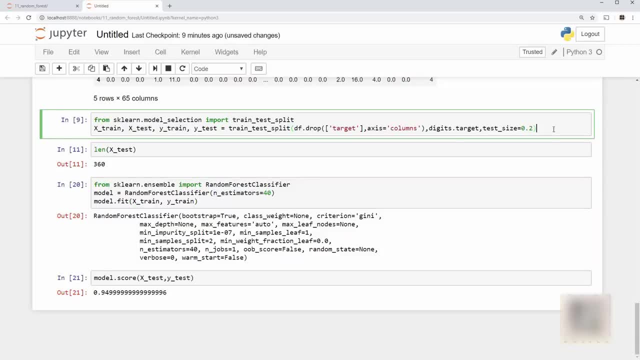 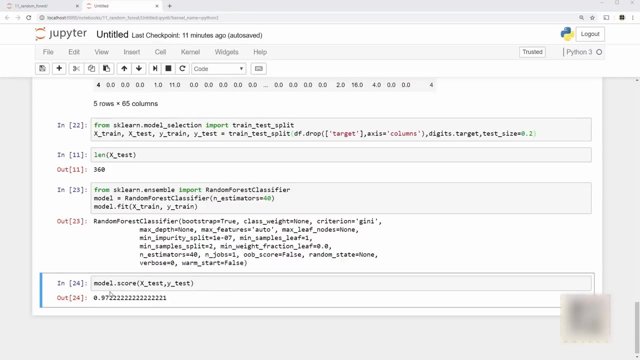 tweaking this parameter. it also depends on your samples as well. so if i execute this line once again, then now my training a set has changed and it might give me a different result. so you see, it perform even better now your model is trained and you can give any sample input, which is nothing. 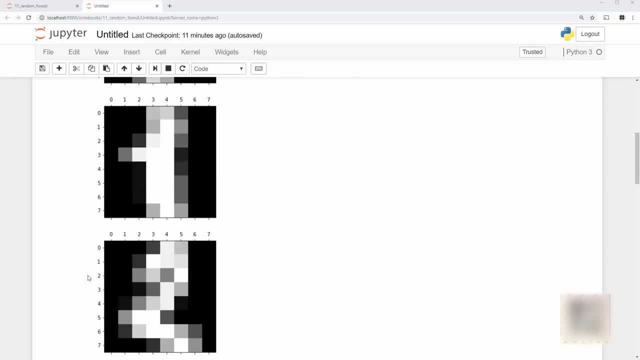 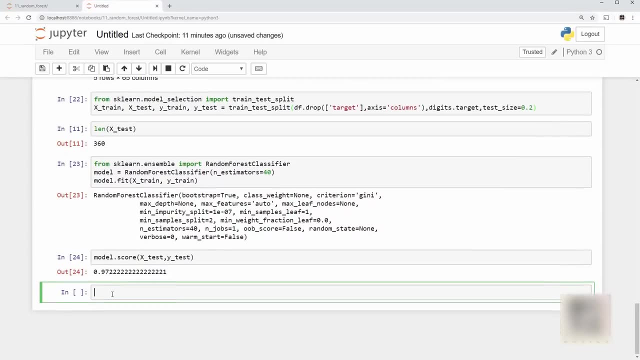 but this kind of henry is actually going to be helping me because i'm adding a different number of trees. this, of course, is because in the test for now i already have the same number of trees, but if i give my model a value of zero, then it will tell me that i can use this particular 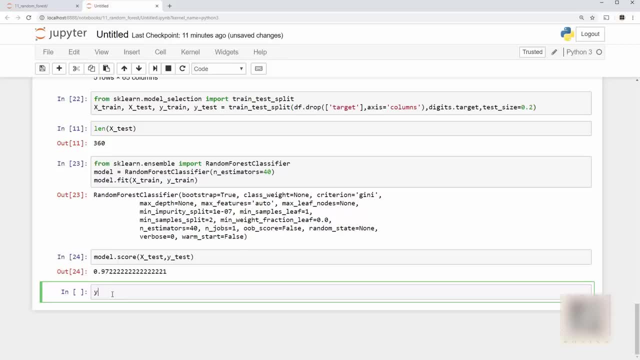 matrix to kind of make a different strength, and then if i create a new model, it will give me the same value. let's see how the model performs. uh, so let's say i create a new model, i want to create a new model. here i'm creating the same model. i can do two additional models. i am just going to. 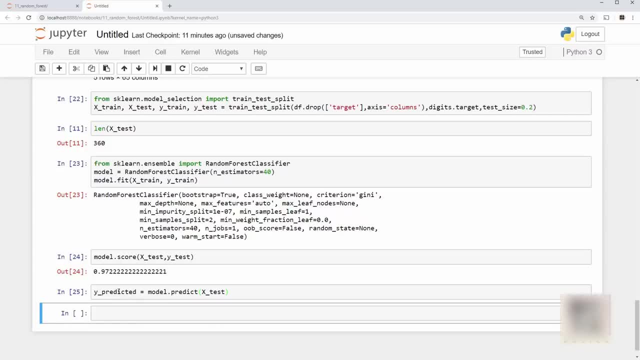 I get Y predicted. this is predicted by model. this is the truth. okay, and confusion matrix allows you to plot truth on one axis and prediction on the other axis from sklearn dot matrix, import confusion matrix and I'm just going to call it CM. here you first supply your truth and then you supply. 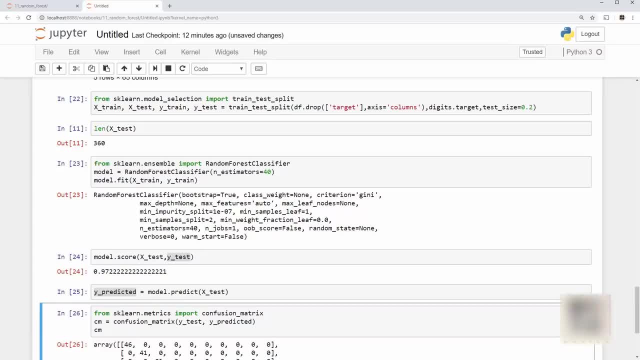 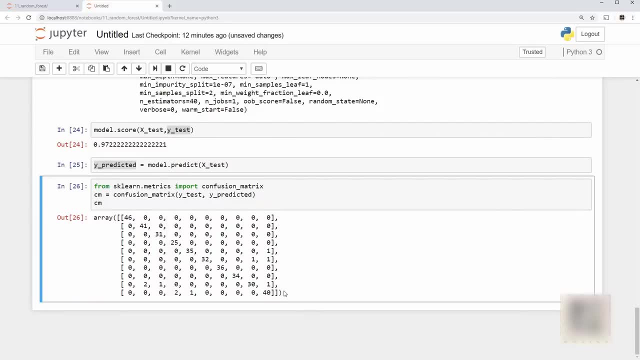 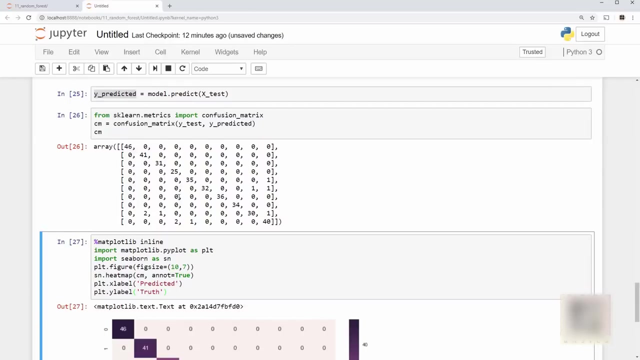 your prediction and when you plot, this is gonna plot two-dimensional array. alright. now this is probably not a better way to visualize it, so I'm going to use a seaborn visualization library. I'm just going to copy paste code just to save some typing. so it's the same confusion matrix, but it's. 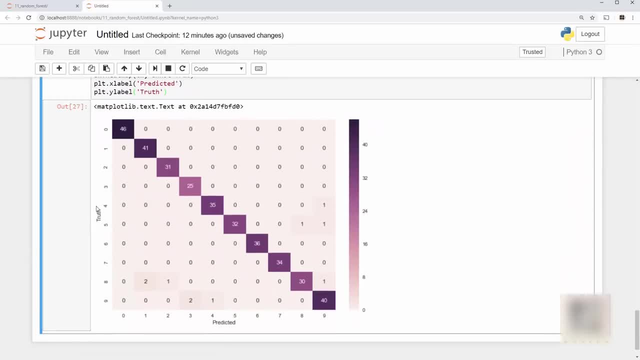 visually more pleasing. okay, so here you have your truth data, you have your prediction, and what this means is I had 46 0 and 46 time it predicted them to be 0, so for 0 it perf. it performed like really well. now what does? what does this? 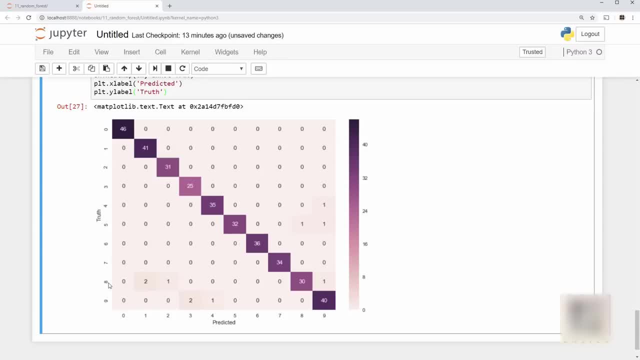 do means this? 2 means I had 2 times the truth was 8, but my model predicted it to be 1, so this is where it made an error: 30 times the truth was 8 and it predicted it to be 8, right. so this, this is a nice visualization which allows you to gauge. 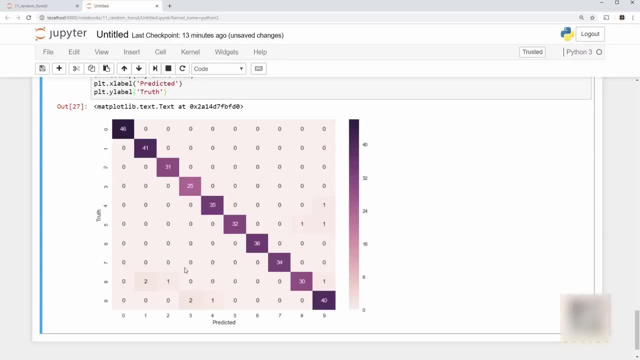 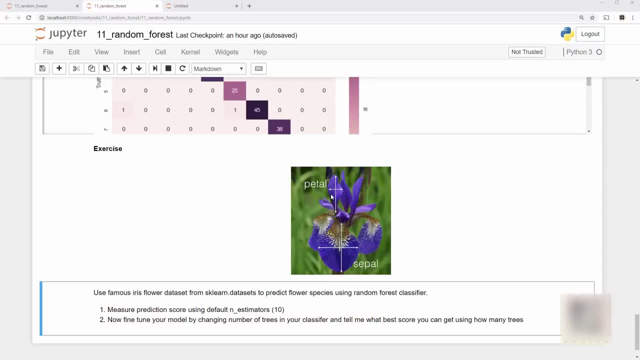 the performance of a model and you should use it more often. all right, now the most interesting part, which is an exercise. we are going to use our famous iris data set from sklearndataset to predict the iris species, and for that we'll use a random forest classifier. so I want you to train your model using the 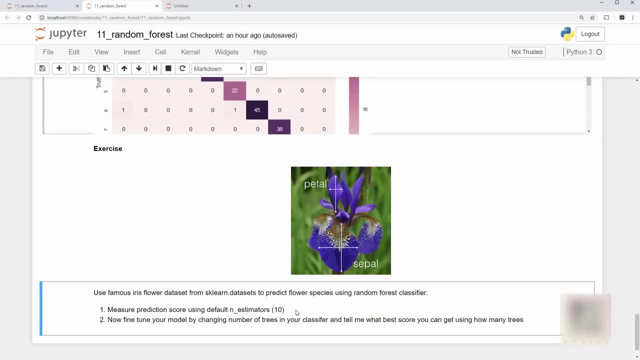 default and estimated parameters and then try to tweak it and tell me what base score you can achieve by using how many trees. all right, you should do this exercise. if you are not going to do this exercise, then you're going to make me very, very angry, all right, so just be afraid of me and just do it.